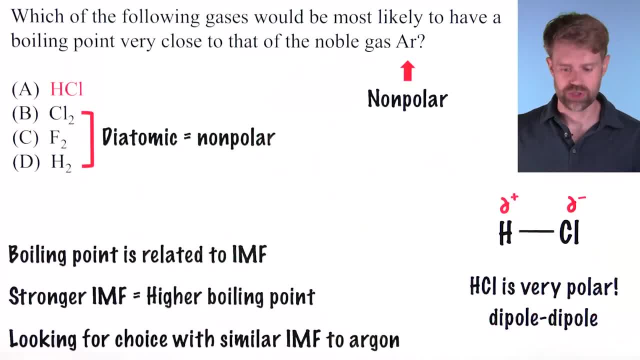 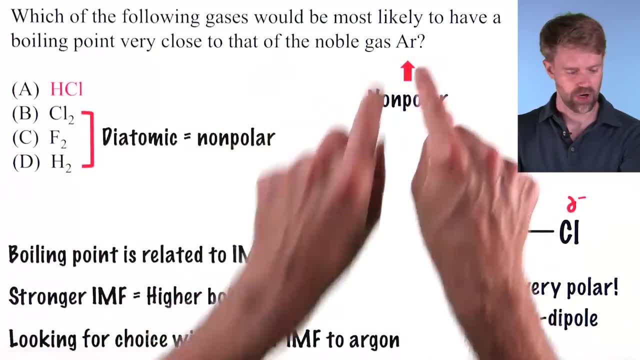 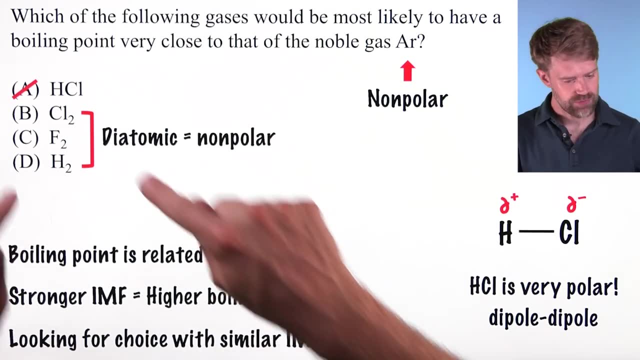 It experiences dipole-dipole attractions which are a strong form of IMF. It's going to have a higher boiling point compared to these and of argon, so we can cross it off. It's the clear outlier. But now we have to figure out which of these remaining three diatomic elements has a similar IMF to argon. 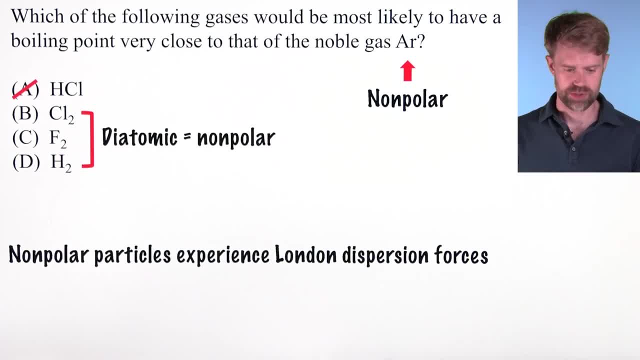 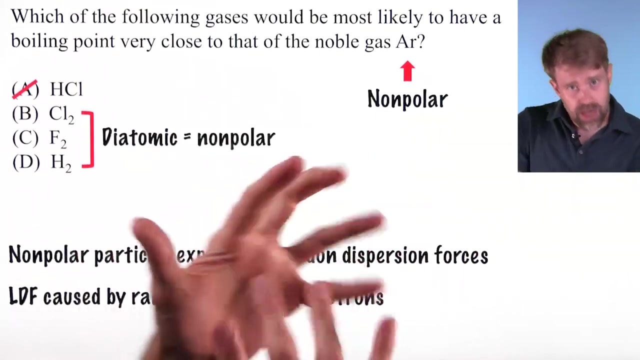 So what kind of intermolecular forces do nonpolar particles experience? Well, they experience London dispersion forces. London dispersion forces, or LDFs, are caused by the random motion of electrons at any given instant. The random movement of electrons creates temporary dipoles, little zones where you have a partial positive and a partial negative charge. 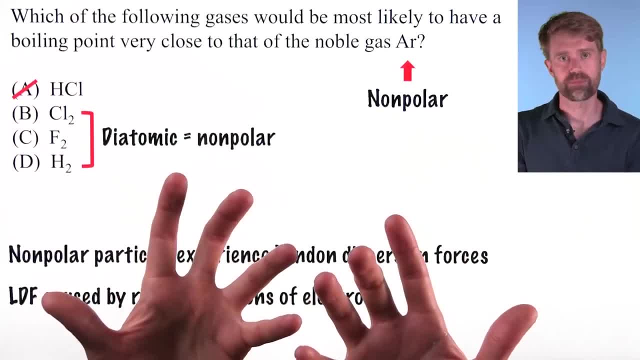 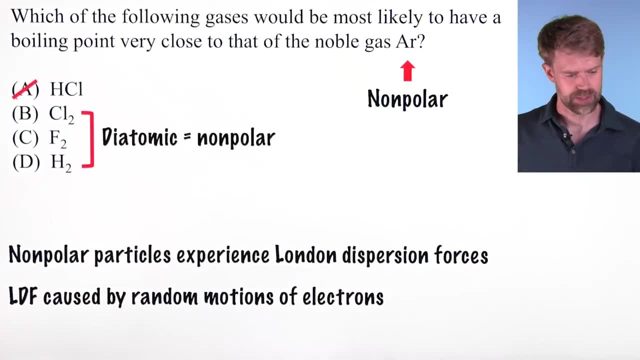 and that creates little flickers of attraction. London dispersion forces are the weakest of intermolecular forces. They're still very important for the AP. So we want to be figuring out which of these molecules has similar London dispersion forces to argon. Well, London dispersion forces are caused by the motions of electrons. 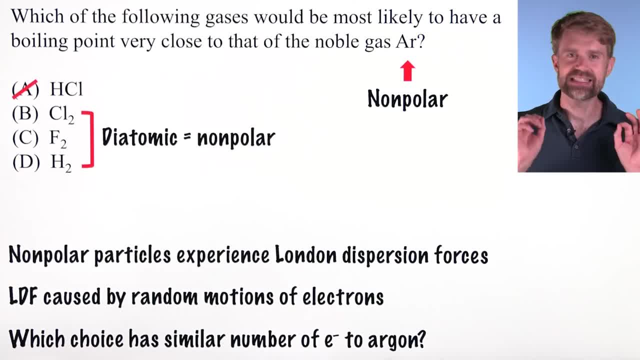 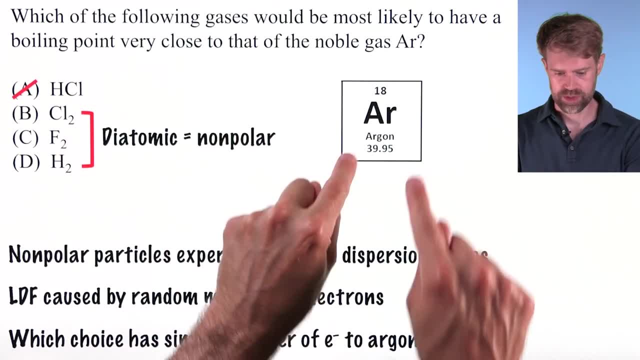 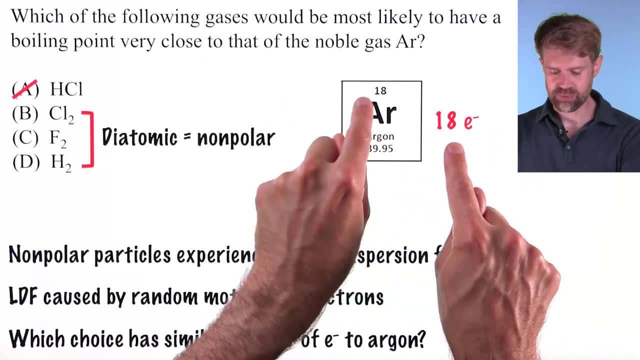 We're looking for an answer choice that has the similar number of electrons to argon. Looking at the periodic table, we see that argon is element number 18.. Because it's electrically neutral, if it has 18 protons it's going to have 18 electrons. 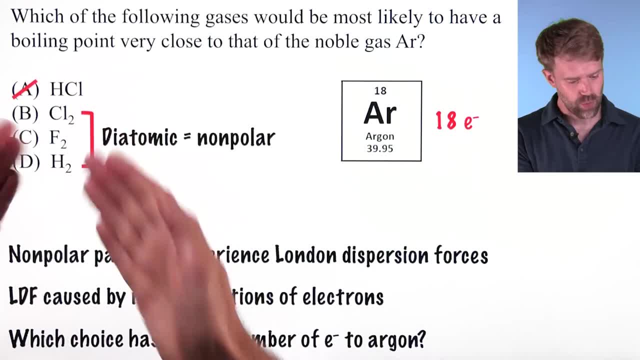 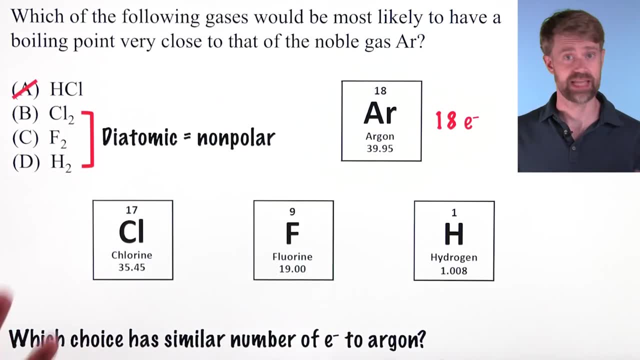 So 18 is a magic number here. Whichever one of these diatomic elements has closest to 18 electrons, that's going to be our correct answer. So let's count up the electrons. We've got chlorine, fluorine and hydrogen. Now, at first you may be tempted to say: aha, chlorine has atomic number 17.. It's got 17 electrons, which is a magic number. Well, that's not true. It's a magic number. It's closest to 18.. 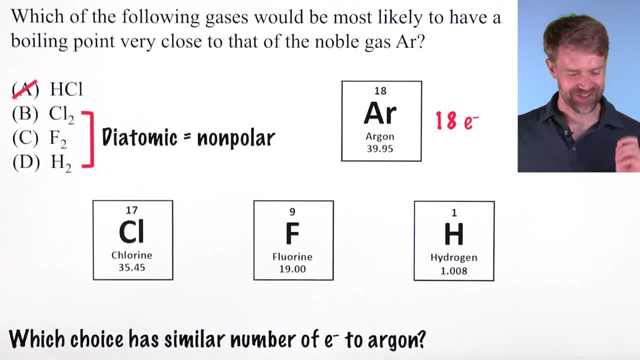 But this is a great example of the AP test trying to trick you Because, remember, these aren't atoms, They're diatomic elements. That means each particle is a molecule of paired atoms: C2,, F2, and H2.. So Cl2 has 34 electrons.